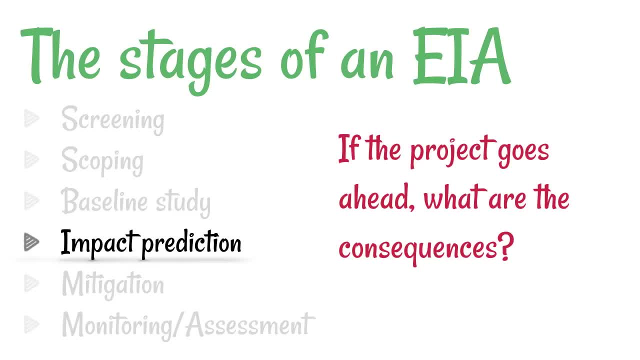 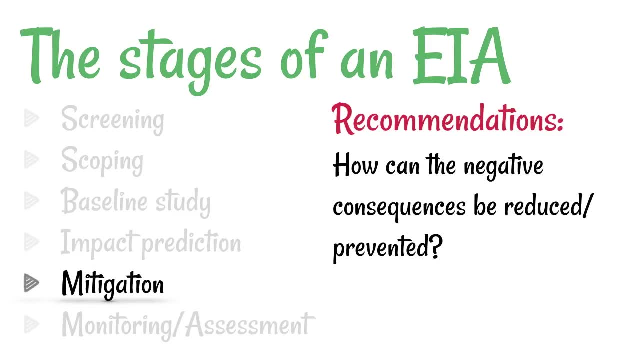 Next is the impact prediction. So, if we do go ahead with this project, what are the possible consequences? And, of course, leading on from that is the mitigation. If we've established what the possible negative consequences are, how could they be reduced or how could they be prevented? 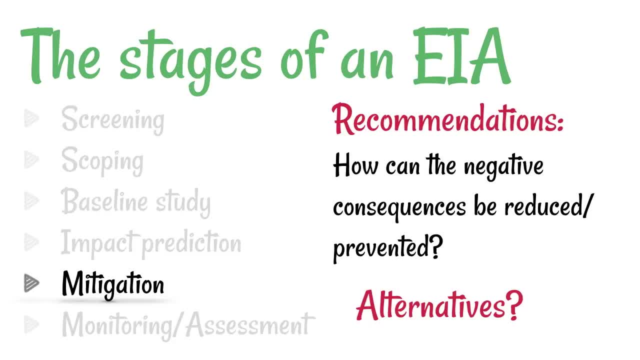 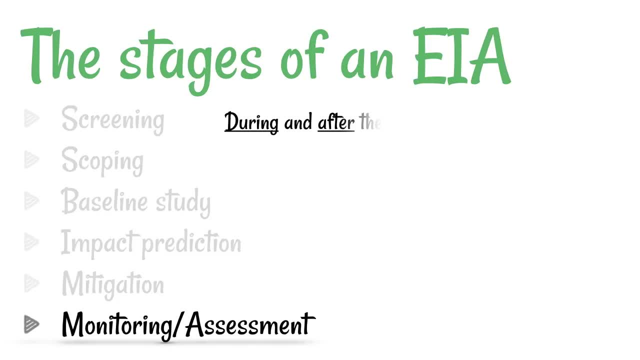 Also, are there any alternatives? So could we redesign the project slightly so that we could then remove these problems? And lastly, there should be adequate monitoring and assessment During and after the project. there should be monitoring of the environmental conditions, which may be continuously changing as the project continues. 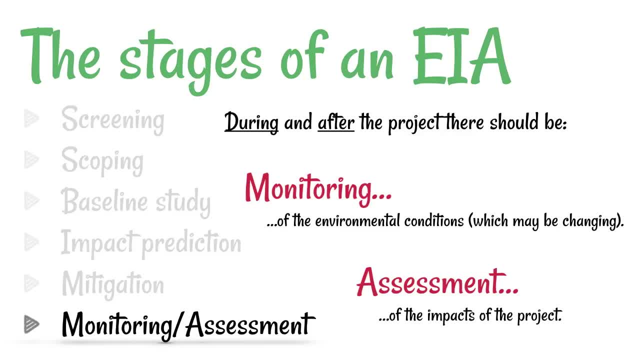 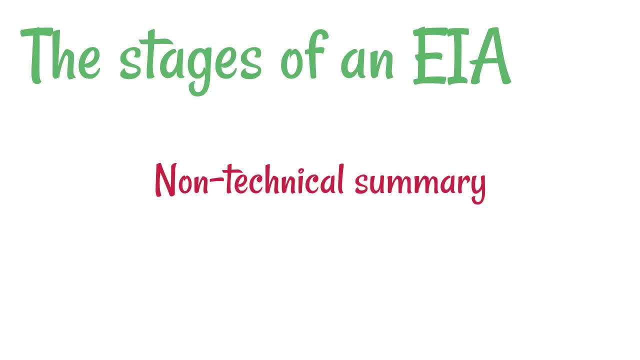 And then, of course, assessment of the impact of the project. The last thing is a non-technical summary. Basically, once this full report, Once this full assessment has been produced, it needs to be presented in a way that non-specialists can understand. 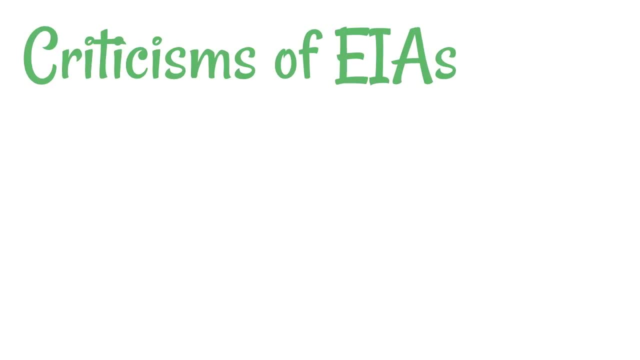 And so that's what a non-technical summary is for. There's a lot of criticisms of EIAs. They're obviously not perfect, Of course. the first one is: sometimes the advice could be ignored. If perfect advice is given on how to reduce the impact, who's to say that that has to be followed? 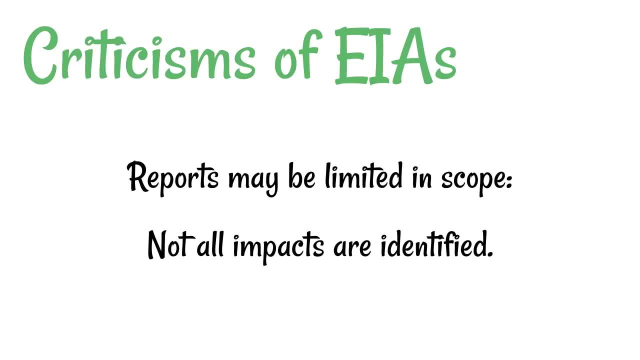 Next, the reports may be limited in scope, meaning all of the potential negative impacts may not have been identified in the first instance. Baseline studies may be incomplete, There might be a lack of available data or, basically, the people who collected the information may not be as knowledgeable about the situation as they need to be. 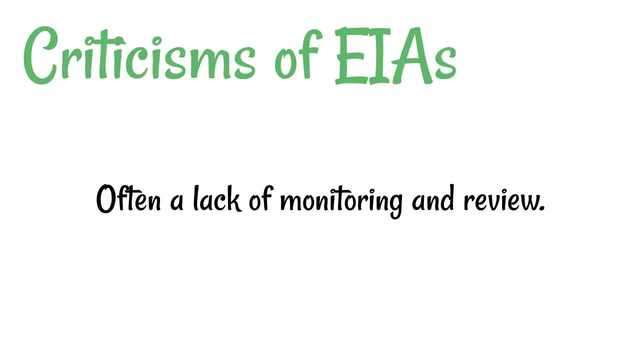 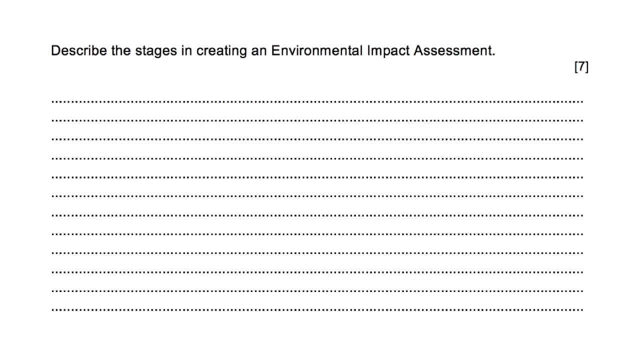 And there's often a lack of monitoring and review. So, basically, once the project gets underway, the negative consequences that develop throughout the project are not always investigated and not always addressed. Let's look at a possible exam question on this. You might get asked. 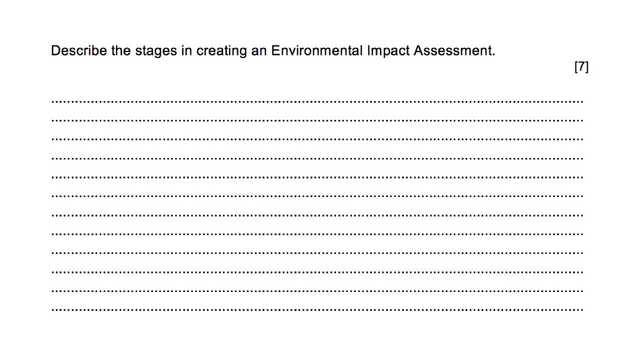 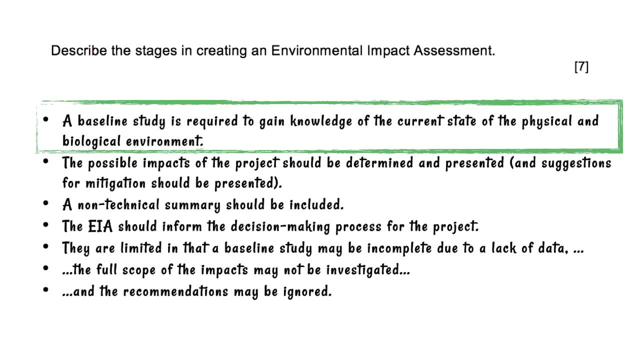 As you can see, it's quite a big question. Seven marks is quite a lot. First of all, your baseline study. Say that it's required and say what it's required for. Next, obviously, the impacts of the project must be understood and this must be presented clearly in the report. 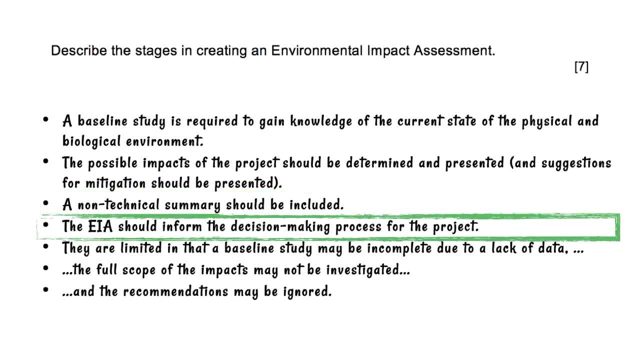 A non-technical summary must be provided, and it's worth mentioning that the environmental impact assessment should inform the decision-making process. You can then go on to describe a little about the limitations. They're limited because the baseline study might not be complete, the full scope of the impacts may not have been investigated adequately and recommendations may be ignored throughout the project.